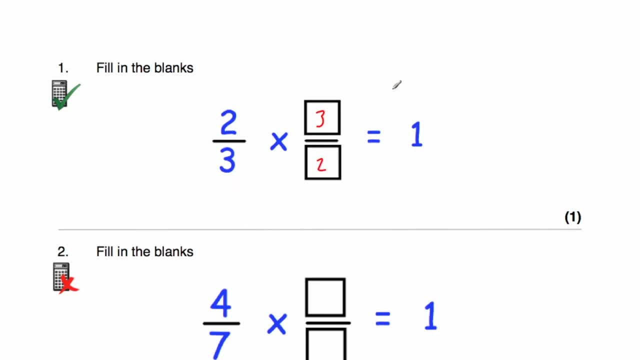 a number multiplied by its reciprocal will always give you one. And let's just check: it's correct. If we had two thirds and we multiply that by three halves, well, multiply the numerators and multiply the denominators. So, multiplying the numerators two times three is equal to six, And three times two is equal to six And six divided. 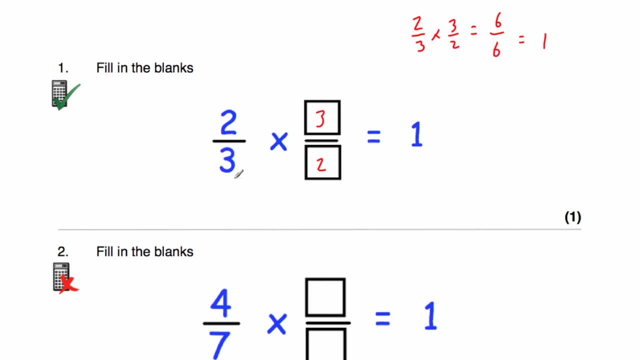 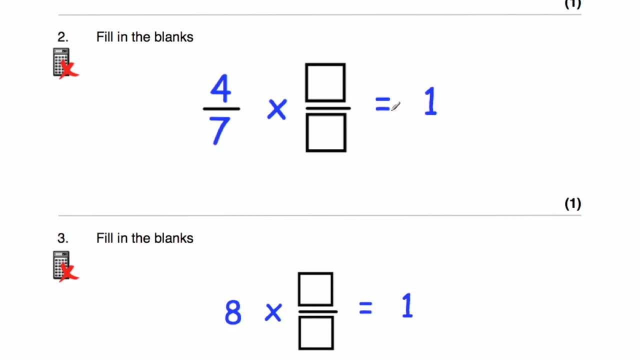 by six is equal to one. So the reciprocal of two thirds would be three halves, And that's the blanks, because the fraction multiplied by the reciprocal will equal one. Okay, question two. Question two: fill in the blanks and we've got four. sevenths multiplied by something will equal one. Well, that's. 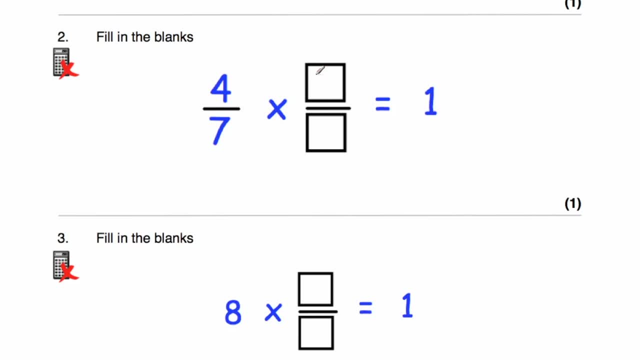 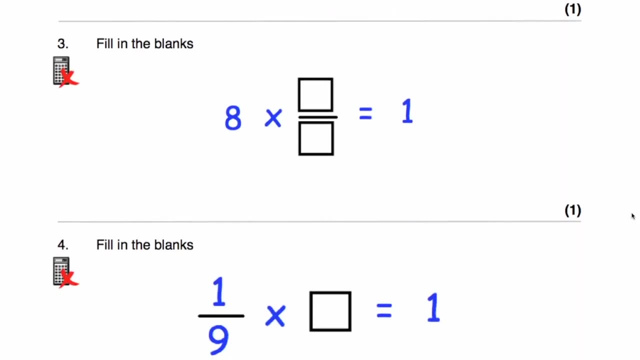 going to be the reciprocal of four sevenths. Well, the reciprocal of four sevenths would be seven quarters, So flipping it over. Okay, question number three. So question number three says eight multiplied by something is equal to one. But if you consider a pizza or a cake and you cut it into, 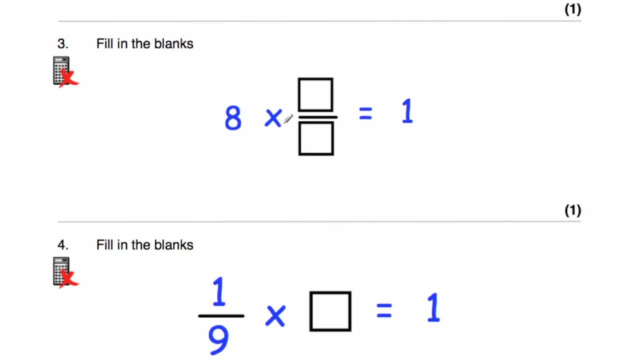 eighths, eight eighths would be equal to a whole. So eight multiplied by an eighth would be equal to one. And if we wanted to get the reciprocal of eight, well, eight is equal to eight over one. flipping it over is: 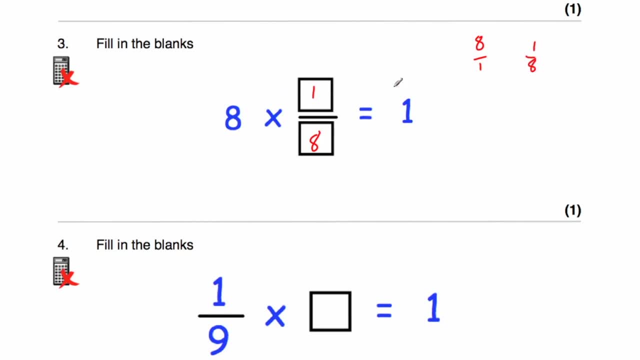 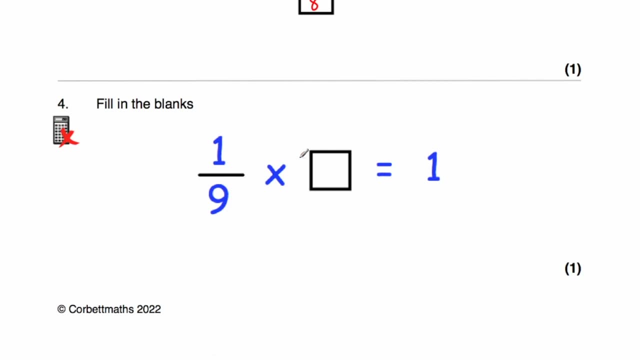 one eighth. So eight multiplied by an eighth is equal to one. So the missing fraction was one over eight. Okay, question four: And ninth multiplied by something is equal to one. Well, if we wanted to make a whole, we would need nine ninths. So a ninth multiplied by nine would be equal to one, And the 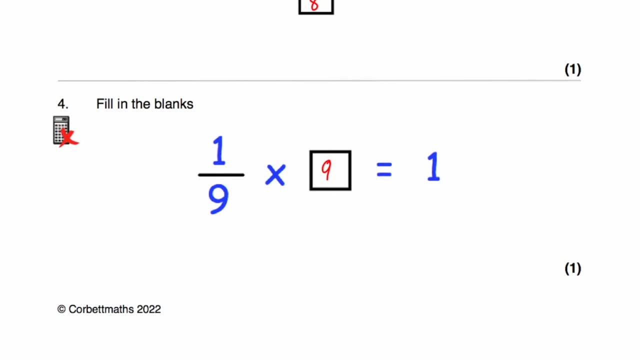 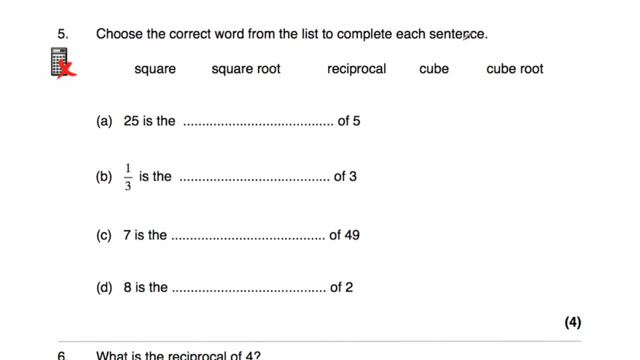 reciprocal of a ninth is nine, nine over one which is nine. Okay, let's have a look at our next question, Question five. So, question five. we've been asked to write in the correct word from the list to complete each sentence. So we've got square, square root, reciprocal cube and cube root, So 25 is the something of five. well, 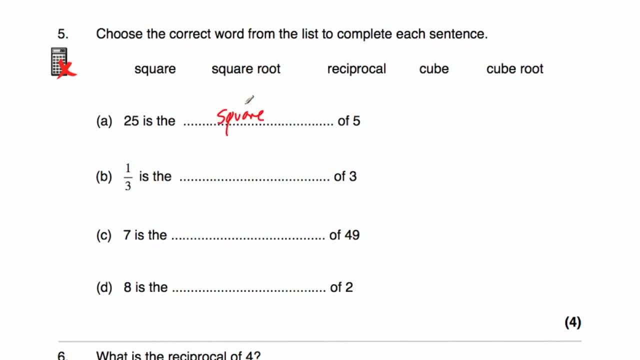 five squared is 25.. So 25 is the square of five, because five squared is 25.. And part B? so part B says the third is the what of three. Okay, so third: well, it's not the square of three, because the square of three is. 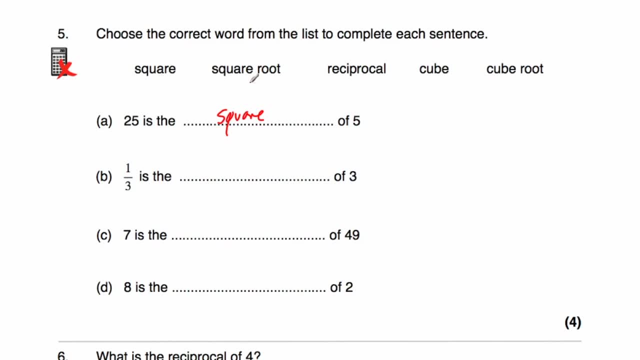 nine. It's not the square root of three, because that's going to be one point something, So it's it's not going to be a third, it's not going to be the cube of three, because three cubed is 27 and it's not. 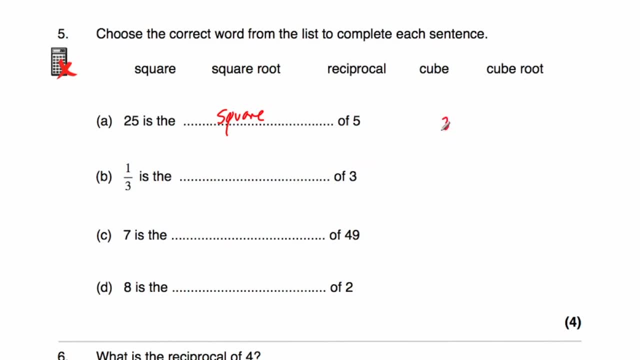 the cube root of three. it's going to be the reciprocal of three, because three is three over one. when you find the reciprocal, flipping it over, the reciprocal would be one third. so it's going to be the reciprocal of three. seven is the something of 49. well, the square root of 49 is seven, so seven. 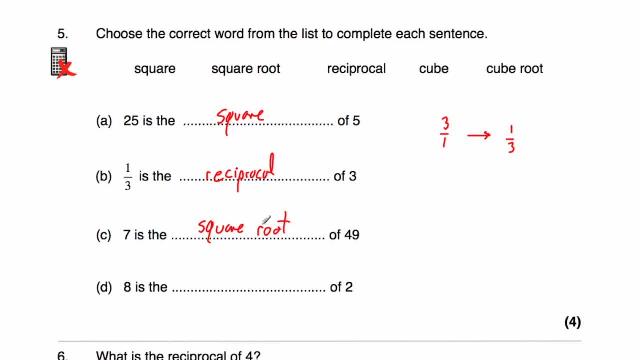 is the square root of 49 and finally, eight is the something of two. well, let's just, we've done square, we've done square root and we've done reciprocal. i'm guessing it's going to be one of these two. not necessarily, i mean, it could be that one of these options is used twice. let's just look. 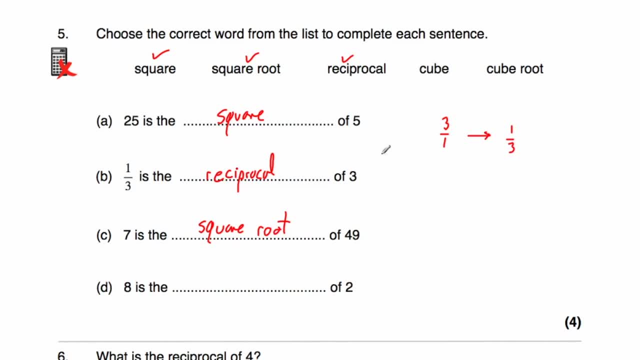 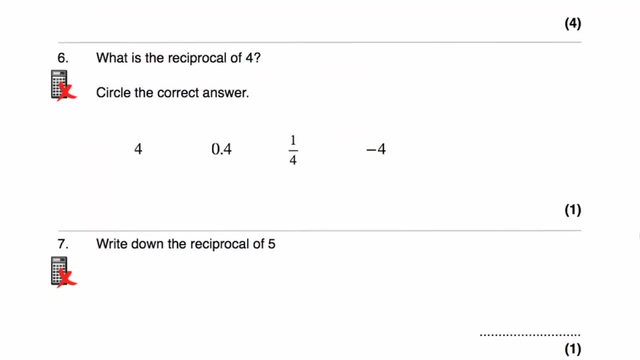 at these. to begin with, it is the what of two. well, two cubed is eight, so it is the cube of two. okay, that's question number five done. let's have a look at question number six. so question number six. question number six is: what is the reciprocal of four? 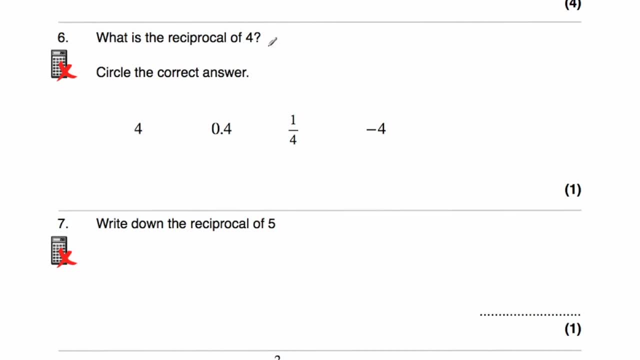 well, what number do we multiply four by to get a whole. but four times a quarter, four quarters as a whole. so the answer would be a quarter, because four times a quarter is one. another way to look at it is if we had four, that's four over one. to find the reciprocal, we flip it over. so that would 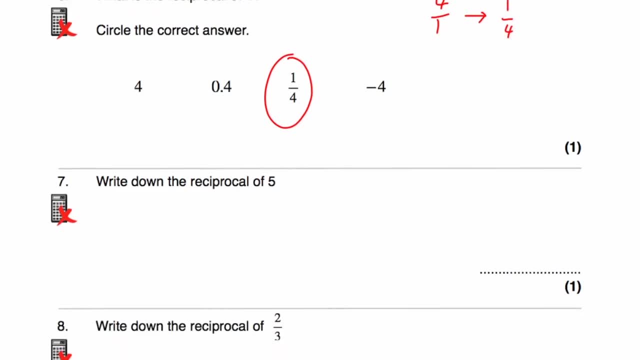 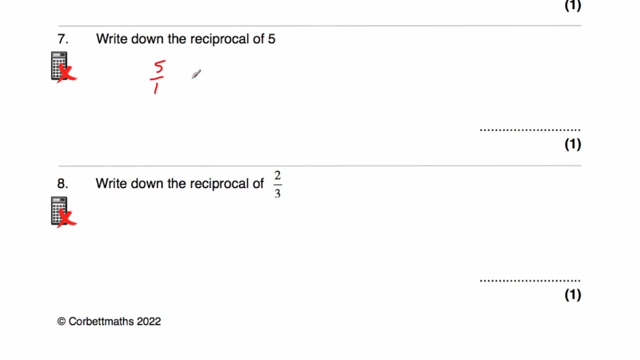 be one quarter. so that would be one quarter, okay. question number seven. question number seven says what is the reciprocal of five? so five of five is five over one, five holes. if we flip that over that's going to be one fifth. so the answer would be one fifth. and just check in, five times a fifth is equal to a whole, okay. 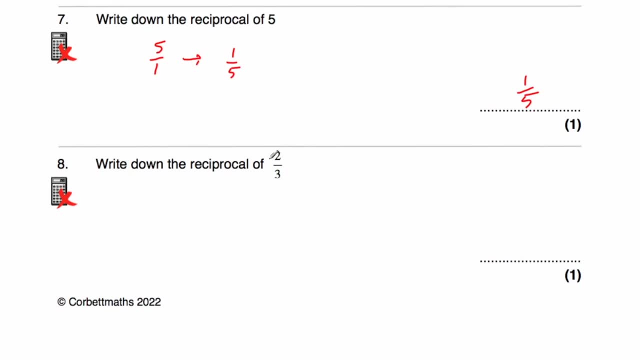 question eight. so question eight says: find the reciprocal of two thirds. well, the reciprocal of two thirds, while flipping it over, would give us three halves, so we could write three halves as our answer. alternatively, we could write it as 1.5, because three divided by two is 1.5, or 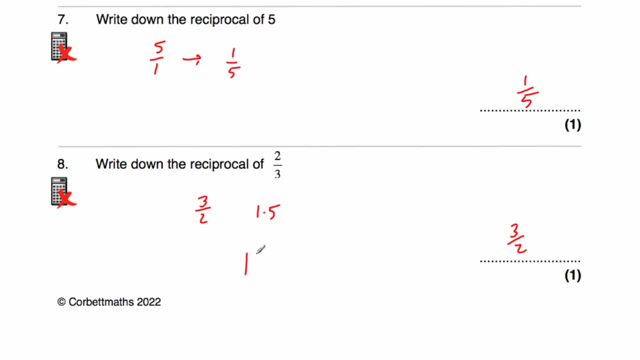 alternatively, we could change it into a mixed number. two into three goes once remainder one and a half, so we can either write our answer as three halves 1.5 or 1.5. okay, question number nine. question number nine says: write down the reciprocal of 10 11ths. 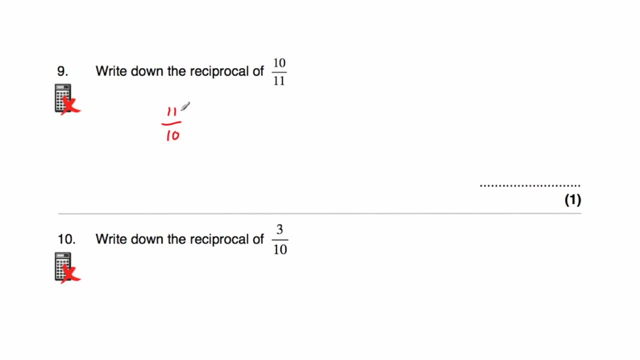 so flipping it over would give us 11 over 10, so that's one possible answer. we could write it as a mixed number, so 10 into 11 goes once remainder one and then the denominator stays the same. so one on one tenth. that could be a possible answer as well. alternatively, we could change our 11 over. 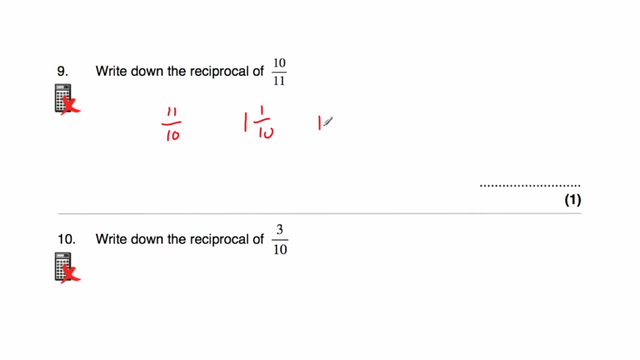 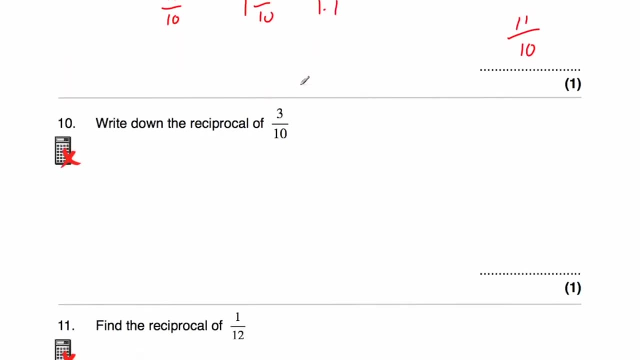 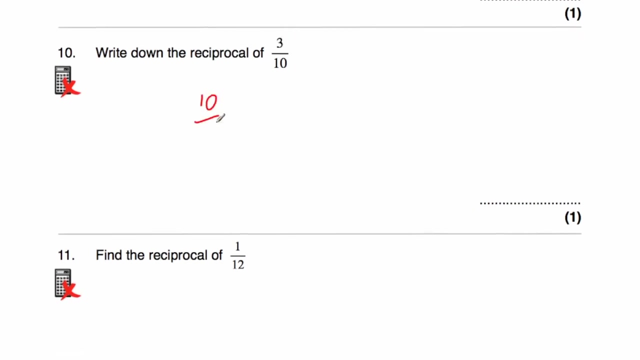 10 to a decimal by dividing 11. divided by 10 is 1.1. so any of those three would be correct. i'm going to write it as a mixed number, okay. question number 10. question number 10 says: write down the reciprocal or find the reciprocal of three tenths. well, three tenths flipping over would be 10 thirds. 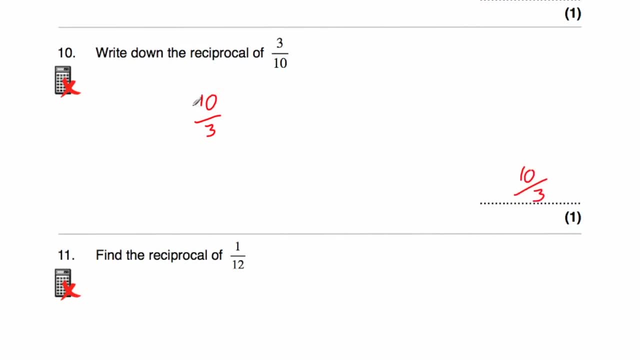 so that could be our answer. 10 thirds- we could write it as a mixed number. three into 10 goes three times. that's nine remainder one and a third. so 10 thirds is three and a third, so that could be a possible answer as well. alternatively, we could change it to a decimal number: three and a third. 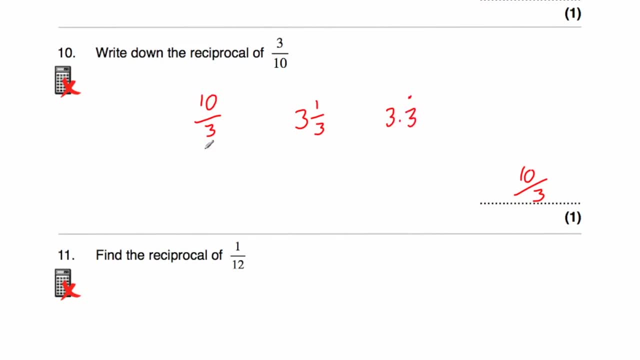 that'll be 3.3 reoccurring. and if you do 10 and a third, that's going to be 10 and a third. so that's 10 divided by three, that's 3.3 reoccurring. i would go for 10 thirds if it was myself, unless i was. 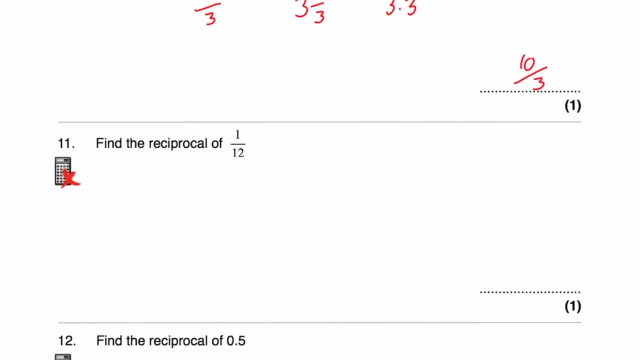 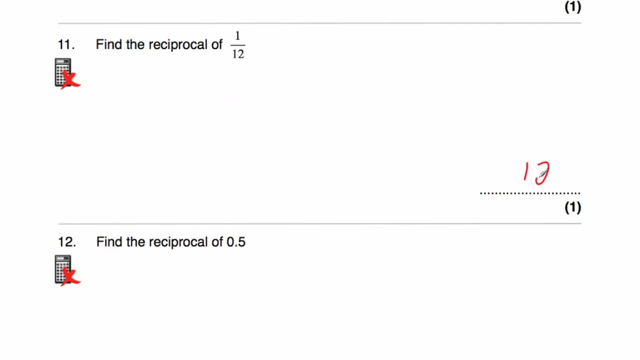 asked to give answers a mixed number or something like that. okay, question number 11. question number 11 asks us to find the reciprocal of a 12th. well, we multiply 12 by 12 to get one, so answer is going to be 12, or another way to think about it is: if we flip it over, we'd get 12 over 1, and that's equal. 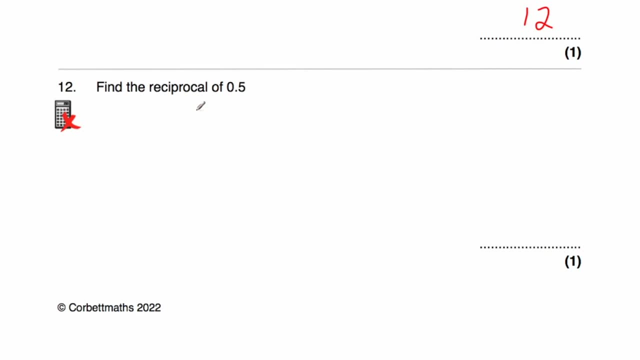 to 12. okay, our next question, question number 12. now, question 12 is a bit different because we've been asked to find the reciprocal of a decimal number. so if you're asked to find the reciprocal number, it can be quite useful to change it to a fraction. so we've been asked to find the reciprocal. 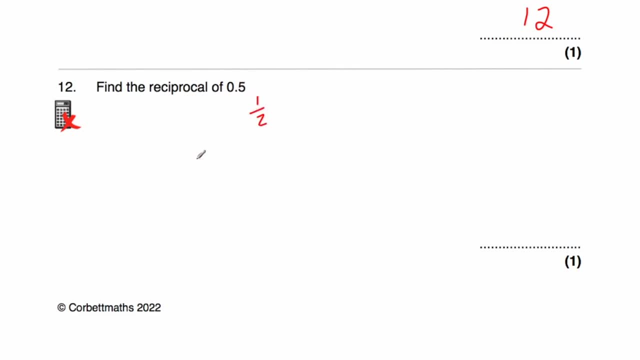 of 0.5. well, that's a half. so we've been asked to find the reciprocal of a half. flipping it over would be 2 over 1 and that's equal to 2. so the reciprocal of a half is equal to 2. so it means: 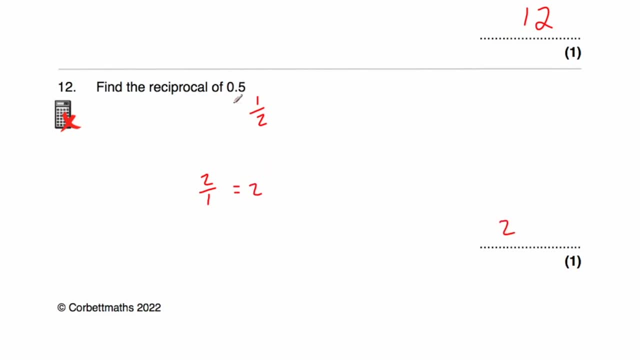 the reciprocal of 0.5 is equal to 2. another way to think about it is: what would we multiply 0.5 by to get 1? and that answer would be 2. okay, our next question, so question number 13. question number 13 asks us to find the reciprocal of 0.5. 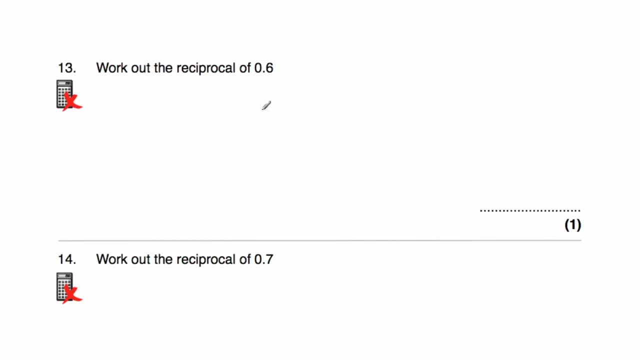 again, this is a decimal number, so it'd be quite useful to change this into a fraction. now, whenever I look at 0.6, I automatically think 3 fifths, because 0.6 is 3, fifths because 1 fifth is 0.2. 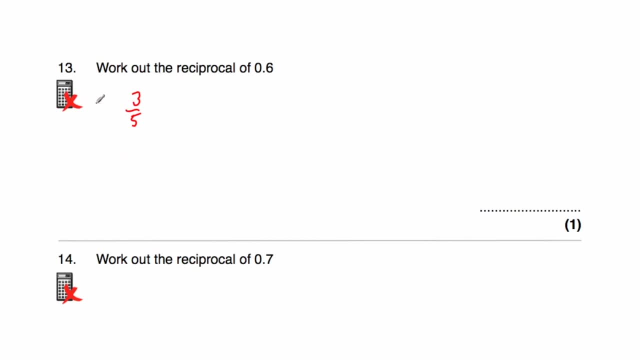 2 fifths would be 0.4. 3 fifths would be 0.6. so 0.6 is equal to 3 fifths. another way to look at it is this is: this is our ones, or our units. then we've got our decimal point. then we've got our tenths. 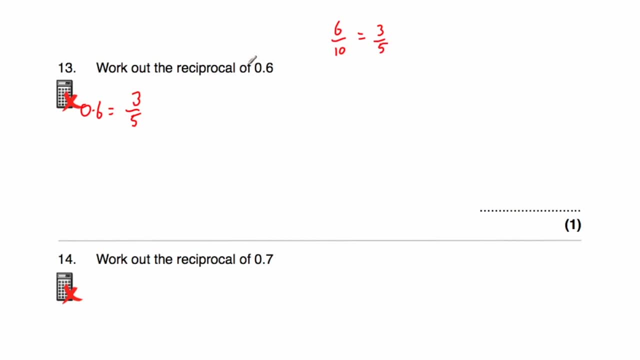 so that is 6 tenths, which would cancel down to 3 fifths. so 0.6 is 3 fifths and we want to find this reciprocal. so we want to flip it over. we want to find this reciprocal, so that would be 5 thirds and that means that our reciprocal of 3 fifths would be. 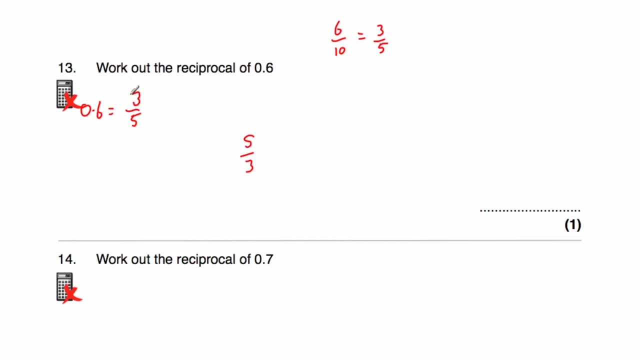 5 thirds. and that also means remember that if we multiply 3 fifths by 5 thirds, we would get 15 fifteenths, which is 1. okay, so the answer would be 5 thirds. we could write it as a mixed number. so 3 into 5 goes, once remainder 2. so 1 and 2 thirds would also be a possible answer, or we: 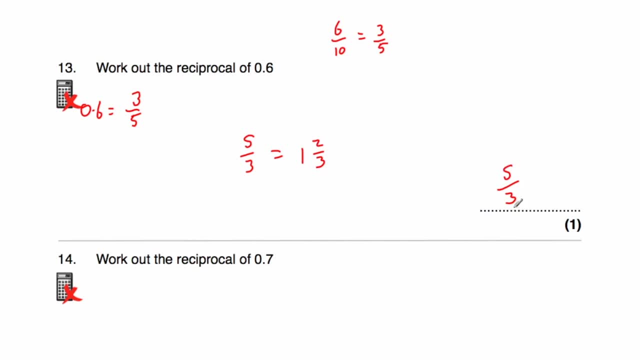 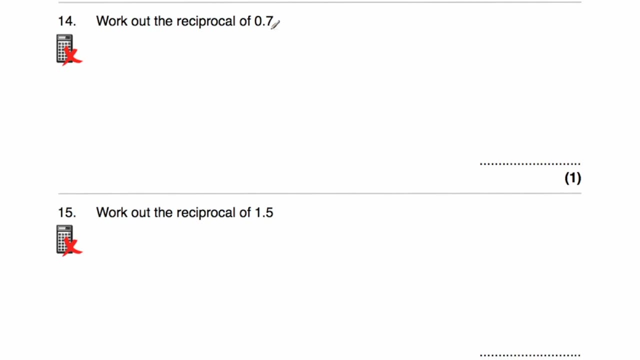 could write it as 1.6 reoccurring, but I would usually give it as a, as a fraction, unless it was asked to give it as a decimal. okay, question number 14. so question number 14 asks us to find the reciprocal of 0.7, so that is 7 tenths, so that's going to be 7 over 10, and finding the reciprocal. 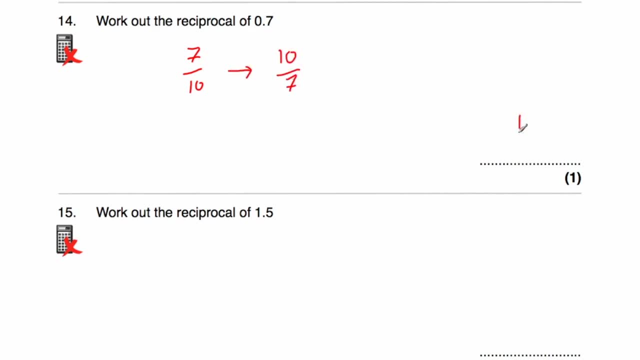 flipping it over would be 10 over 7. so the answer would be 10 sevenths and if we multiply these two numbers together, our 7 tenths. what we were given are 0.7 or 7 tenths by 10 sevenths. that would be: 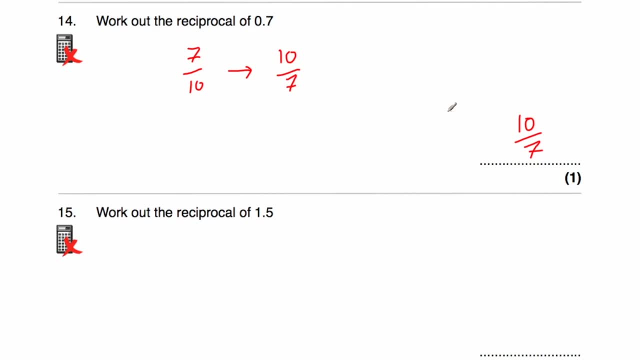 70 seventieths, which is 1. also remember we could give our answers a mixed number and that would be 7. into 10 goes, once remainder, 3 over 7, so you could give it a 7 tenths, or 1 and 3 sevenths. 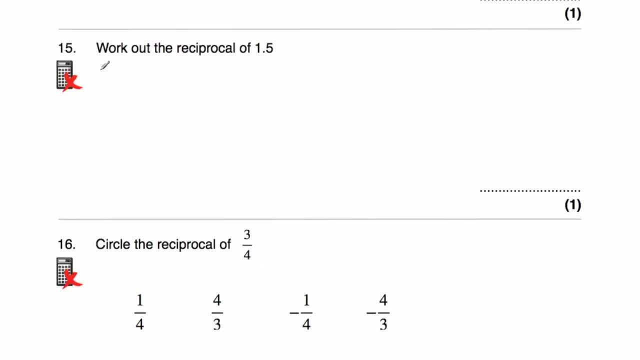 okay, question number 15. so question number 15. question number 15 asks us to find the reciprocal of 1.5. so whenever I'm finding the reciprocal of a number, I prefer it to be a fraction, so I can just flip it over nice and quickly and easily, and if it's a mixed number I like to have that as a top. 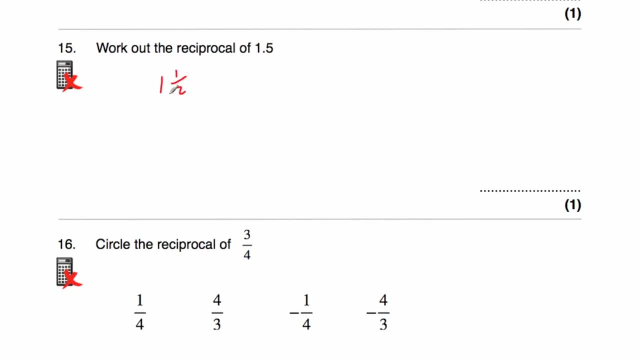 1.5. because it's 1.5, 1.5, I do like to have it as a top every fraction before finding the reciprocal. so changing our 1.5 into a top every fraction: 1 times 2 is equal to 2 plus 1 is 3. so 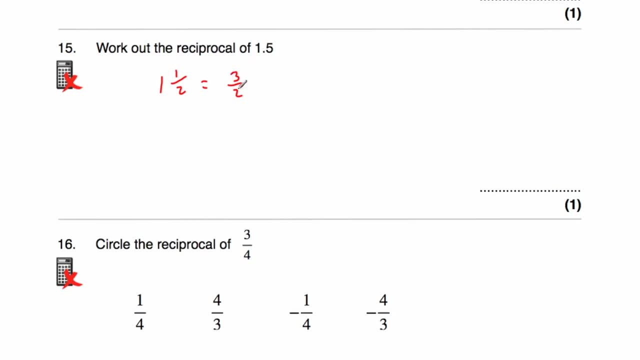 that would be 3 over 2. so 1.5 is three halves. and then I want to find this reciprocal. so three halves, flipping it over, we give us two thirds. so that would be two thirds. so I changed the 1.5 into a. 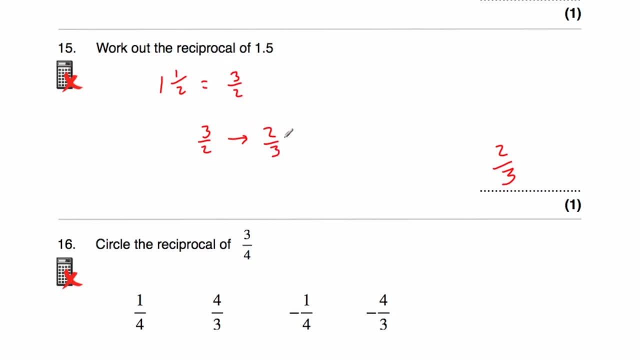 top every fraction, three halves, and then I just flipped it over to get two thirds. and let's just check our answer: if we had three halves and we multiply it by two thirds, three times two is equal to six. two times three is equal to six. that's six sixths, which is a whole okay question. 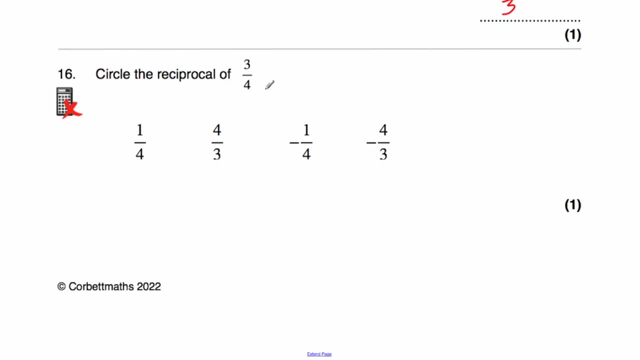 number 16. question number 16. we've been asked to circle a reciprocal of three quarters, so the reciprocal of three quarters flipping over would be four thirds and our options are: a quarter no, four thirds yes, minus a quarter no and minus four thirds no. okay, question number 17. so question. 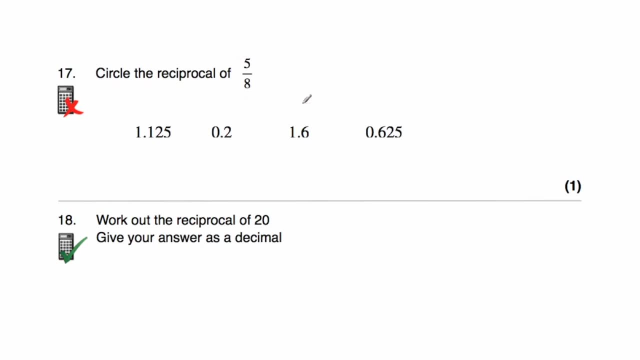 number 17 asks us to circle the reciprocal of five eighths. interestingly, here we've got our options, but they're all decimal numbers, so we're going to need to find the reciprocal and then convert it into a decimal number. so, five eighths: finding the. 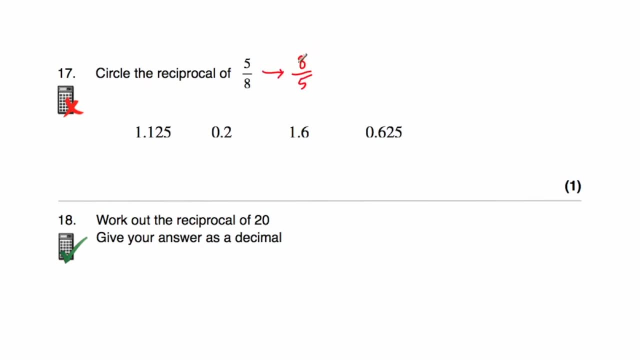 reciprocal flipping it over would be eight fifths now, eight fifths we. we don't have that on the list, so we need to convert that into a decimal number. so let's do to change a fraction to a decimal. we can divide the numerator by the denominator. so if we do eight divided by five, we will find what. 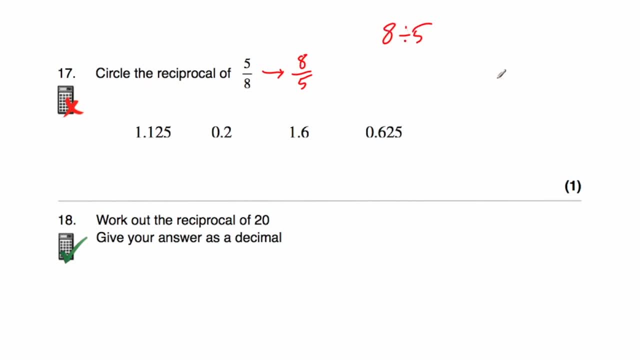 our answer is- and it's a non-calculator question- so we're going to do eight divided by five. so dividing eight will go under the bus shelter. the number we're dividing by will go in front and let's do short division to work out our answer. so eight divided by five. well, let's put a decimal. 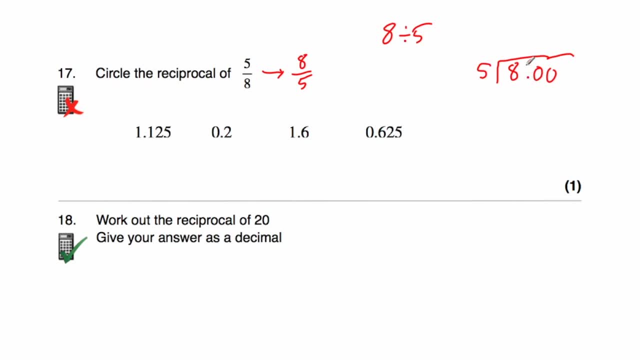 point in some zeros, just because we know that it's going to be a decimal answer, and let's put our decimal point above. so, eight divided by five. well, how many fives go into eight? that's one, remainder three, so put it there. how many fives go into thirty? that's six and no remainder. so answer. 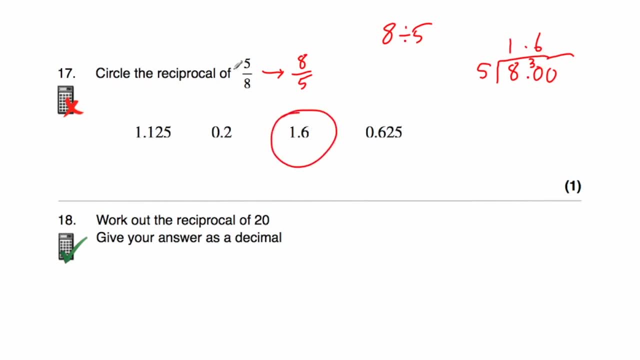 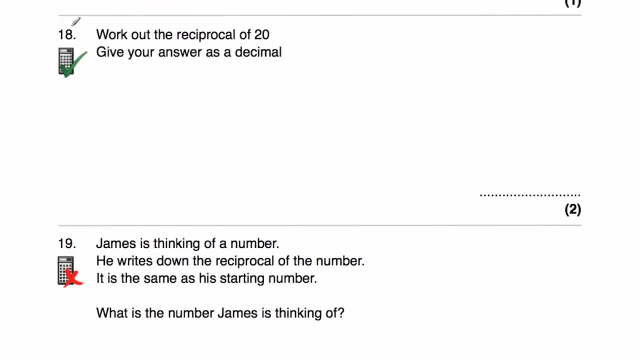 is 1.6 and, as you can see here, we've got 1.6 as an option. so that's our answer. so the reciprocal is 20.. okay, our next question, so question number 18. question number 18 says: work out the reciprocal. 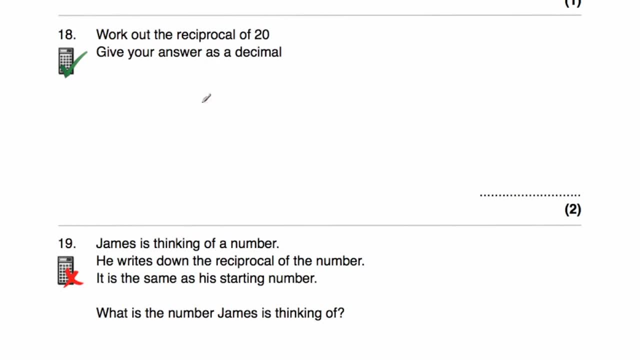 of 20 and we're to give our answer as a decimal. so let's find the reciprocal of 20. so if we have 20, which is the same as 20 over 1, and we want to find this reciprocal, we flip it over, so that'd be 1- 20th. 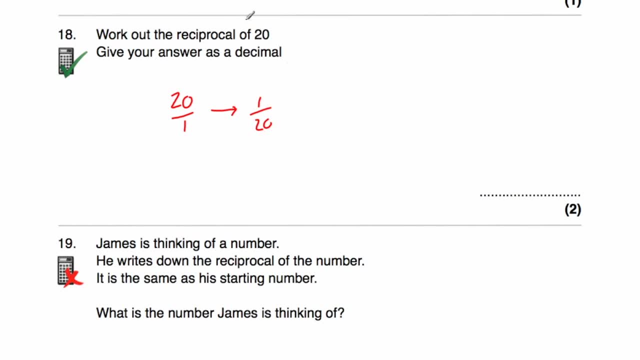 so the reciprocal of 20 is 1- 20th and that makes sense. what number g times 20 by to get one? well, that'd be 1 20th if you had 20 20ths. that's a whole and we're to give our answer as a decimal. 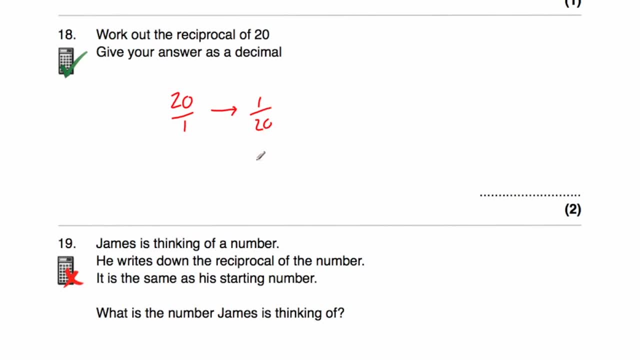 number and that's a calculator question. so you could just do one divided by 20, on the other hand, the calculator and change that into a decimal and that should give you 0.05. or if you don't have a calculator, like the way I've just done that in my head was I know that 1 10th is equal to 0.1. so 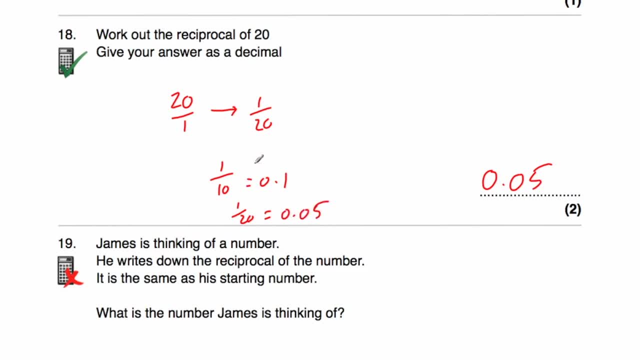 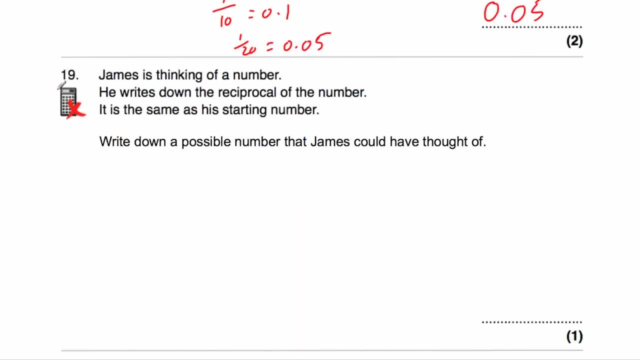 1, 20th would be half that, which would be 0.05. but it is a calculator question. so you should be organized and have your calculator and do 1 divided by 20 and it gives you 0.05. okay, let's have a look at question number 19. so question number 19 says James is thinking of a number. 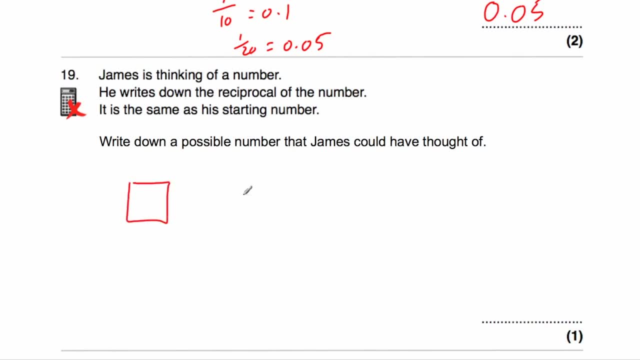 so James is thinking of a number and he writes down the reciprocal of the number. so he writes down the reciprocal of the number. so he writes down the reciprocal of the number. so he writes down the reciprocal of the number and it's the same as the starting number, so that 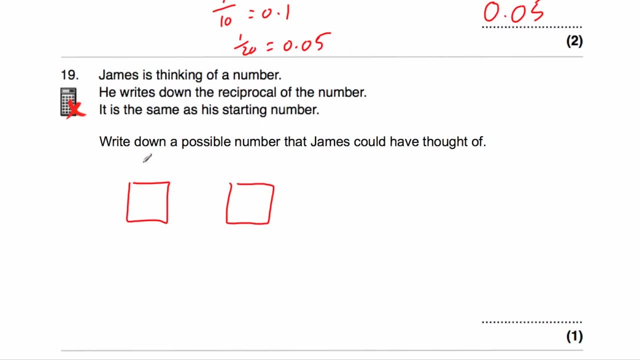 means that his reciprocal is the same as the number he started with. we've been asked to write down a possible number that James could have fought off, so we know that the number and its reciprocal are the same as each other, and we're trying to find what number that is. so we know that. 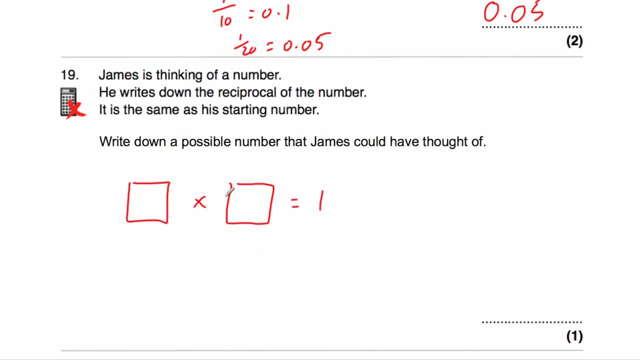 a number multiplied by its reciprocal will always give us one, and we know these two things are the same. so we're trying to find the number that, when we multiply by itself, it would give us one. so we've got two possible options here. we can have one times one, because one times one is equal to one. 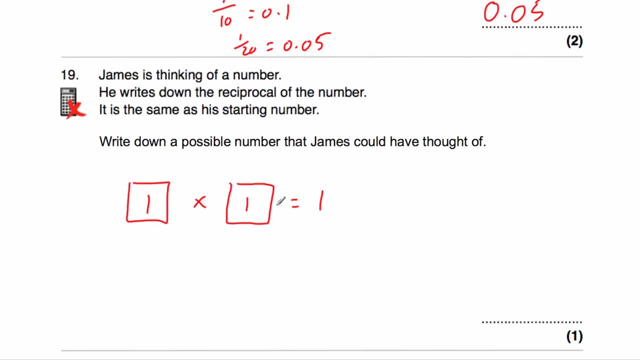 so that means that if we start with one, the reciprocal of one is one, and that means that one is a possible number that James could afford off. another option he could afford off- well, if we could have started off with a different number. and we still know that these two things are the same and they multiply together to give us one. 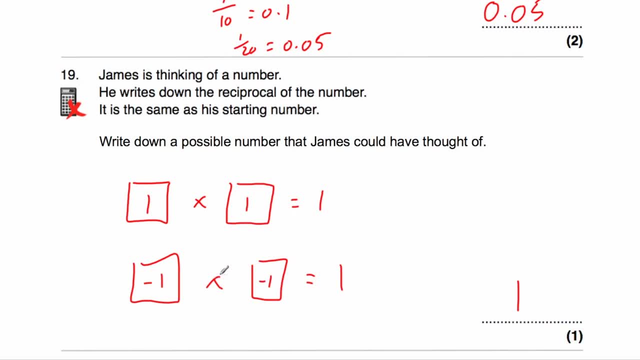 well, another option could be negative one, because negative one multiplied by negative one and negative times the negative is a positive, so negative one multiplied by negative one is also equal to one. so the two numbers the GMS could have fought off could have been one or a negative one. 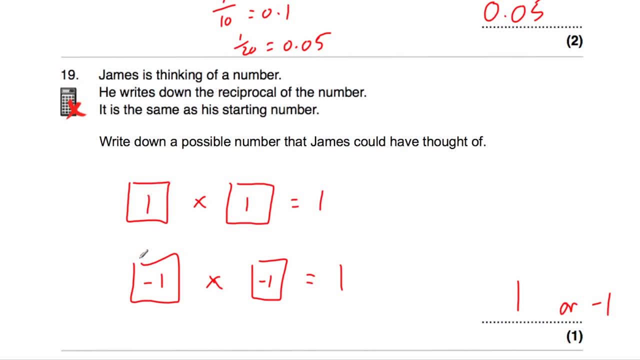 and let's just think about it: the reciprocal of one is one and the reciprocal of negative one is negative. one way we can consider is in terms of fractions. so if we start off with 1, which is 1 over 1, if we find it's reciprocal, flip it over, that's equal to 1 over 1. so you can see they're the same as each. 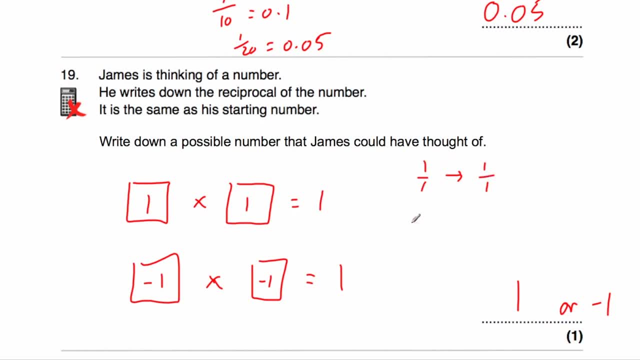 other. so the reciprocal of 1 is 1.. alternatively, if we start off with negative 1, so that's negative 1 over 1 and we flip it over, that would be equal to 1 over negative 1 and if you divide both of. 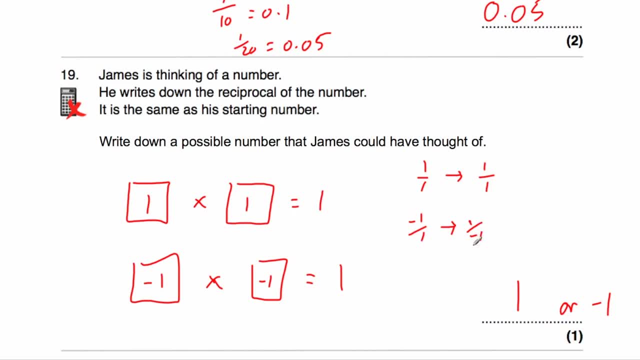 these negative 1 by 1, you get negative 1, and 1 divided by negative 1 is also equal to negative 1, so the reciprocal of one is one and the reciprocal of negative one is negative one. so if you ever ask for a number, that whenever you find it's reciprocal it's the same as its number, the number. 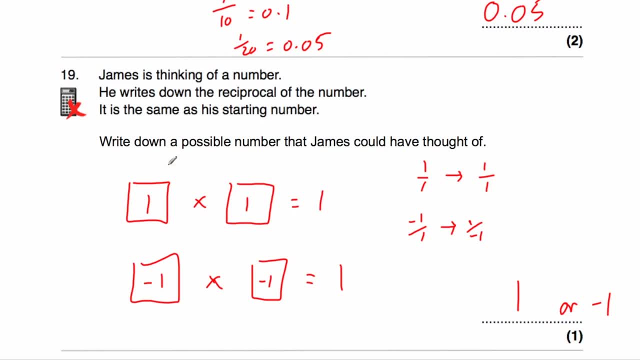 itself. your answers could be one or negative one. now this question just has to write down a possible number that james could afford off. so i probably would just write down one, because it's the one i think of first, but you also could have negative one. okay, let's have a look at our next. 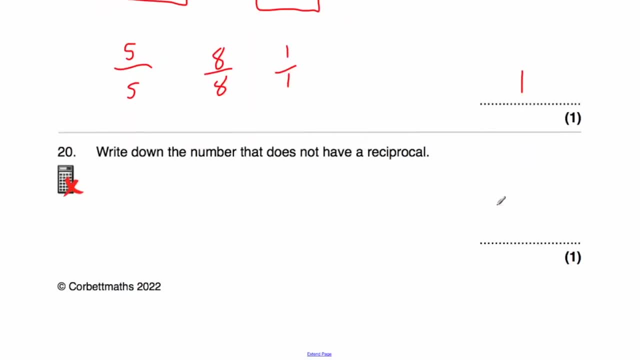 question: okay, question number 20. write down the number that does not have a reciprocal, that's going to be zero, because remember that a number times best reciprocal gives you one. if you have zero and you want to multiply it by something to give you one, there's no number that you can put. 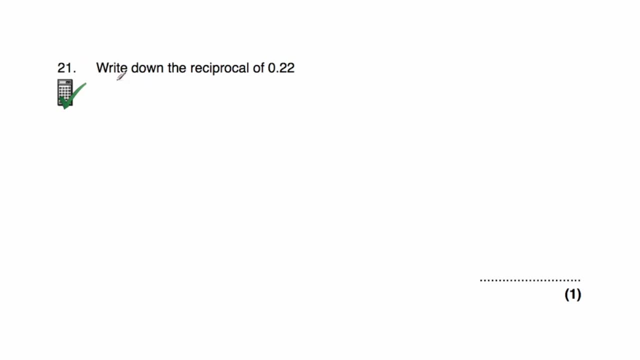 there to give you that. okay. question number 21: it's a calculator question and it says: write down the reciprocal of 0.22. so if you wanted to change 0.22 into a fraction, you could press 0.22 in your calculator and press equals and if it's in the right mode it will give you an answer of 11 over. 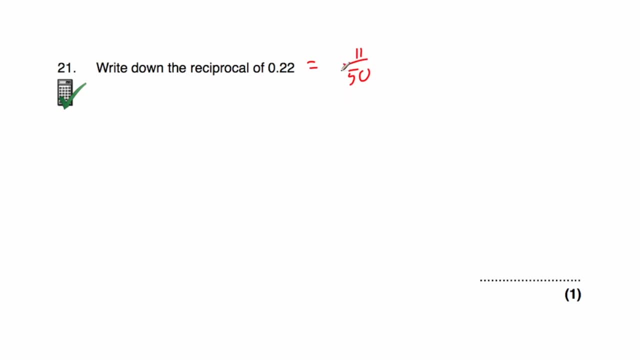 50. so no point two. two as a fraction is eleven fiftieths. if you didn't have a calculator to hand it a handy, if that was a non-calculator question, you could say: well, that's twenty two hundredths, because obviously you've got units, or ones tenths and hundredths. 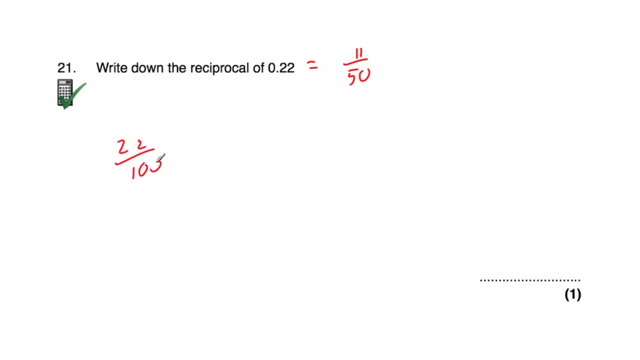 that's twenty two hundredths, that's twenty two over one hundred, and if you cancel it down that's eleven fiftieths. but because it's a calculator question, we could just type in 0.22, press equals, and it will give us our fraction as long as your calculator is in the right mode. so we've got eleven. 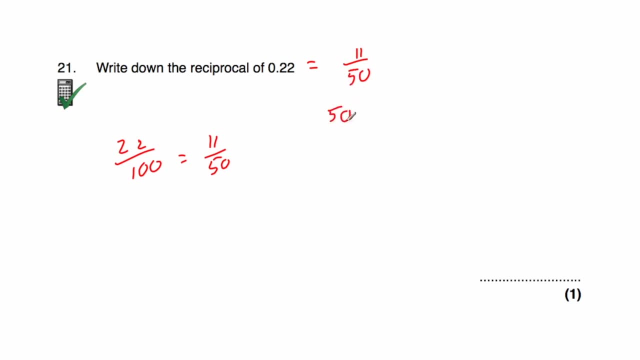 fiftieths- we want to find this reciprocal, so that's going to be flipping over- would be 50 over, so the answer would be 50 elevenths. alternatively, we could change it to a mixed number if we wanted to. how many elevens go into 50? well, four of them is 44, so it's 4: 44. remainder 6 over 11.. 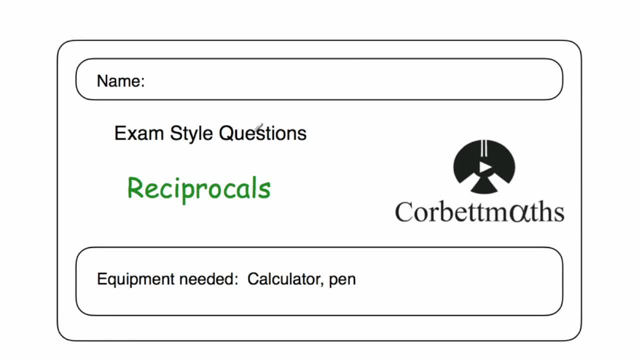 so either of those answers would do, and that's it. so these have been the video solutions to the reciprocals practice questions. i really hope you found this video useful. if you have found it useful, please like it, please subscribe to the youtube channel and if you do need any extra, 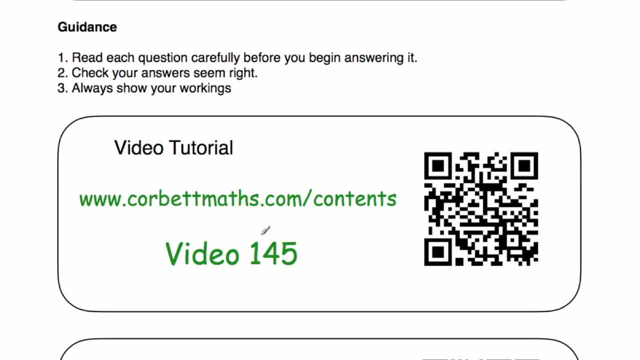 help on the reciprocal. if you go to codemavscom forward slash content, so scroll down to video 145 or scan this qr code. that will help you okay, thank you, cheers bye.